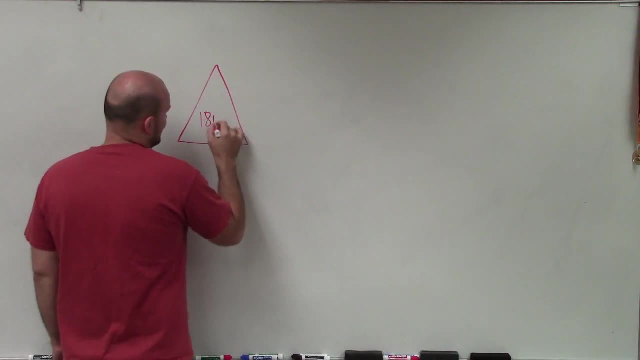 of interior angles of a triangle is going to be 180 degrees, So that's going to be kind of like our given. It doesn't matter what the triangle looks like. It doesn't matter if it's a isosceles like this, It doesn't matter if it's an equilateral, which would 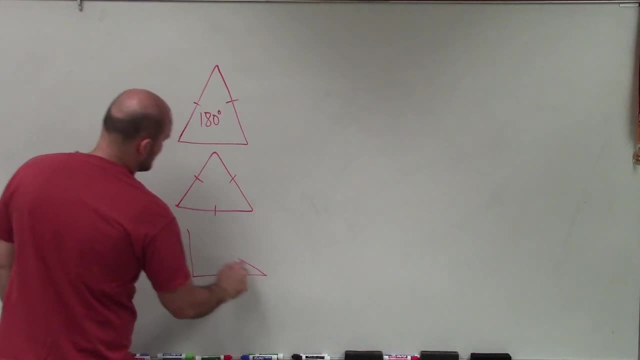 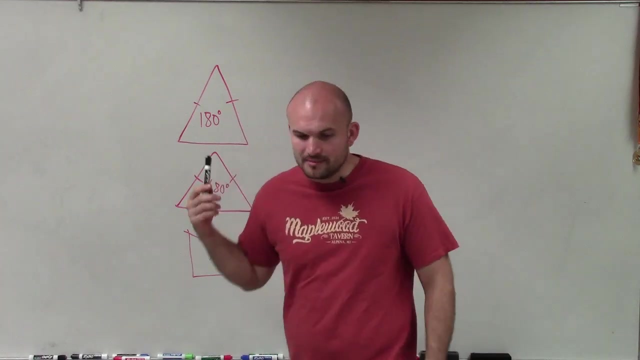 be a regular triangle, which we're going to use very often, or if it's a right triangle, All the angles, the sum of all these angles, is always going to equal 180 degrees, So we're going to use that definition to help us identify what is going to be the sum of all the angles. 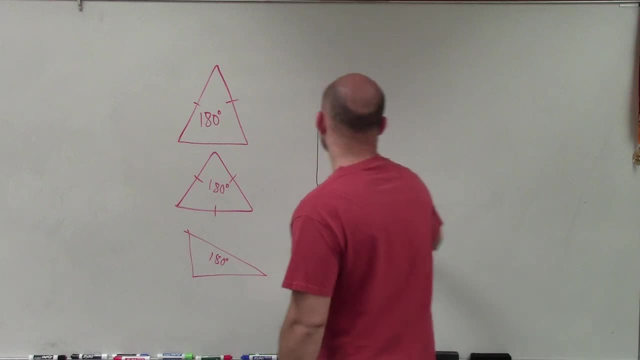 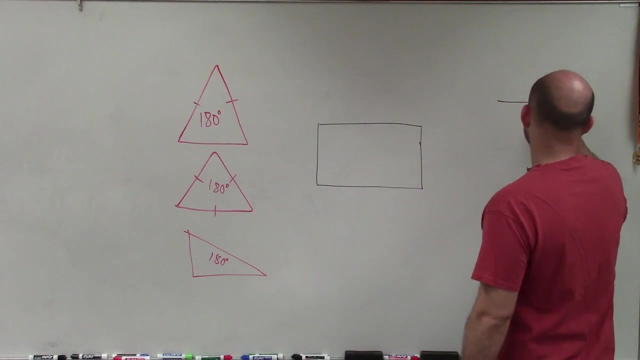 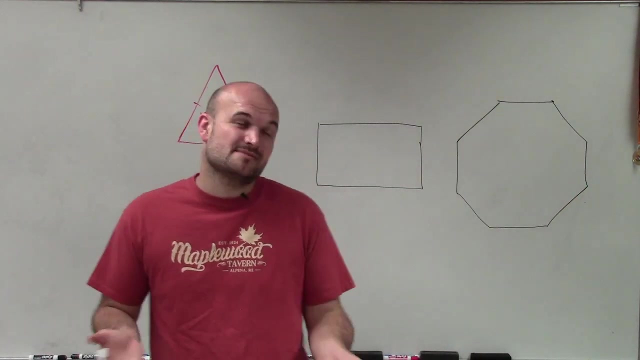 in any type of polygon, And so I'll go and look at a rectangle which would be a quadrilateral or a regular octagon, And I'll try to do my best creating a regular octagon, But so when you're trying to determine the sum, it doesn't. 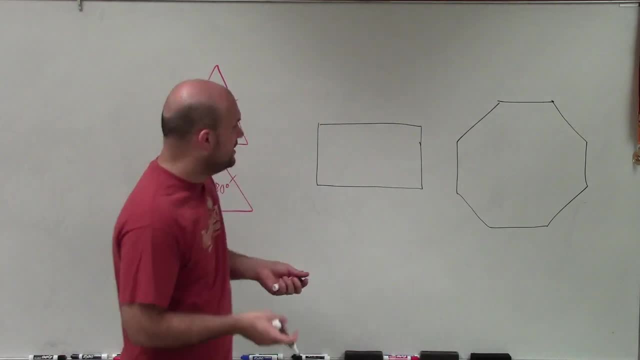 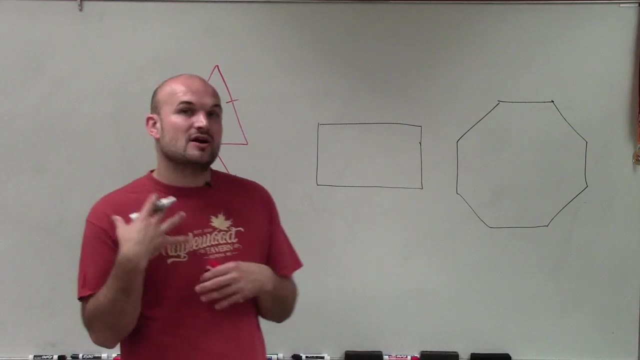 matter if it's regular, meaning all the angles or all the sides are exactly the same- But it does have to be concave. It cannot be a convex polygon. It can only work when it's concave, as far as at least the process that I'm going to show you. So the way that we're 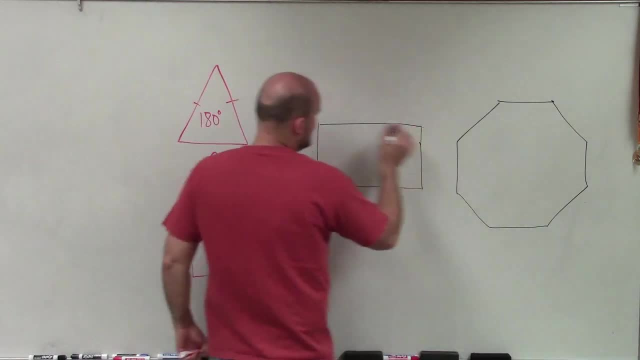 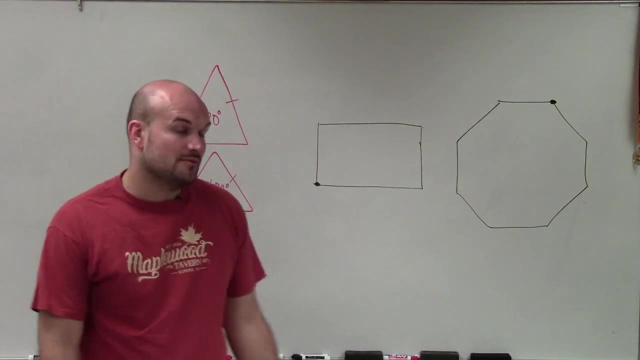 going to do this is: we're going to choose a vertex And you can see that each where, and it doesn't matter where you choose your vertex, But you're going to select a vertex. Then what you're going to do is you're going to draw a line to every other vertex. Well, 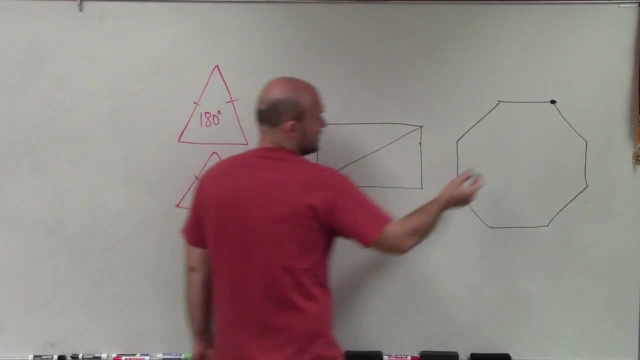 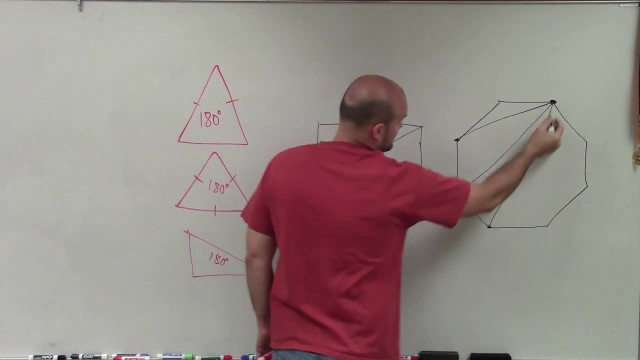 I already have a line here, So now I'm simply going to draw a line there. Here I can draw a line to this vertex line, to this vertex, line to that vertex, line to that vertex and a line to that vertex. Now all I'm simply going to do is count the number of triangles. 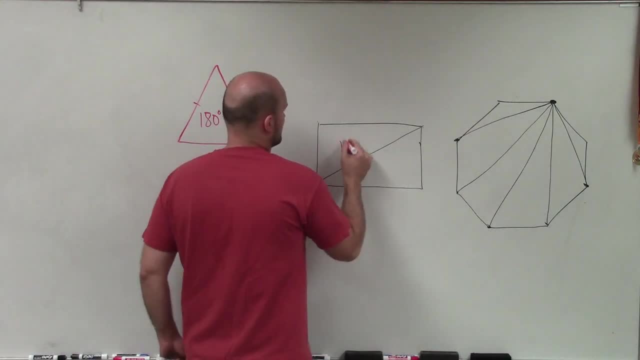 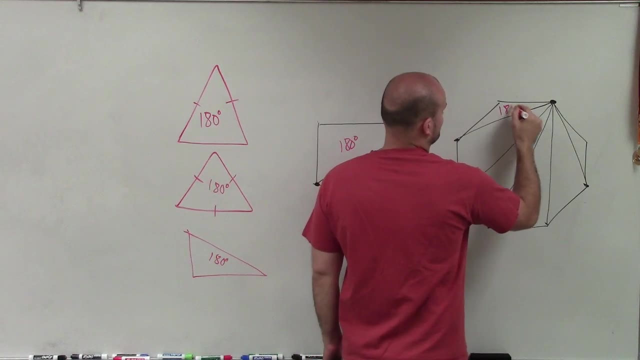 that I have And you can see, here I have two triangles: 180 degrees, 180 degrees, 180 degrees. Here I have 1,, 2,, 3,, 4,, 5, 6.. So there, I have six sides. Now there's an important. 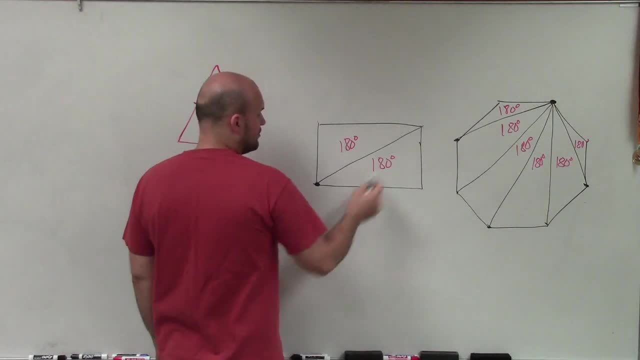 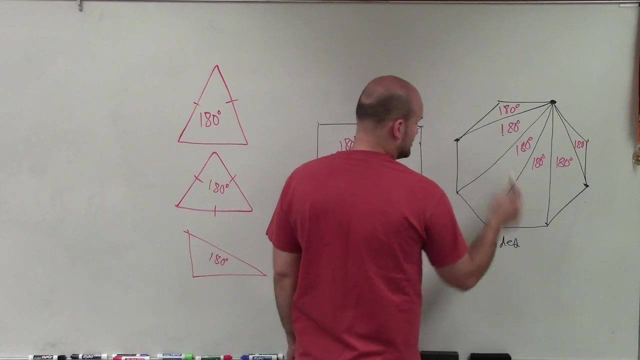 thing to notice and to understand. So, when we look at this, the number of sides is equal to 4.. The number of triangles is equal to 2.. Here, the sides are equal to 8. And the triangles is equal to 6.. And if you repeat this for